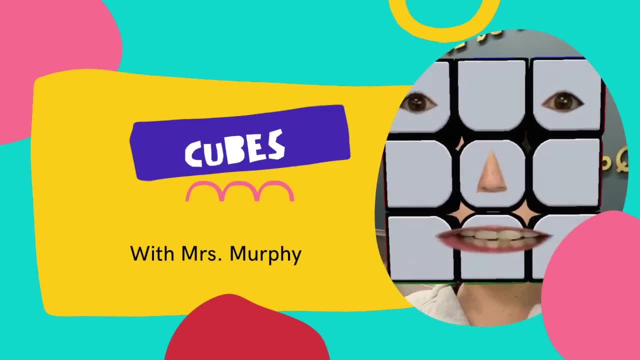 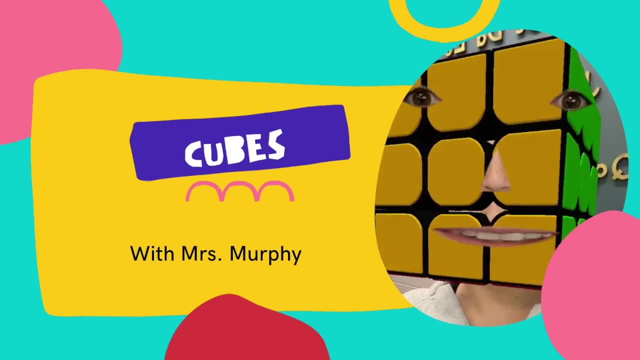 Hey friends, Today we're going to learn about another 3D shape. Can you guess what shape we're going to learn about? We're going to learn about cubes. In this lesson you'll learn the attributes of a cube. Then you'll practice finding cubes amidst. 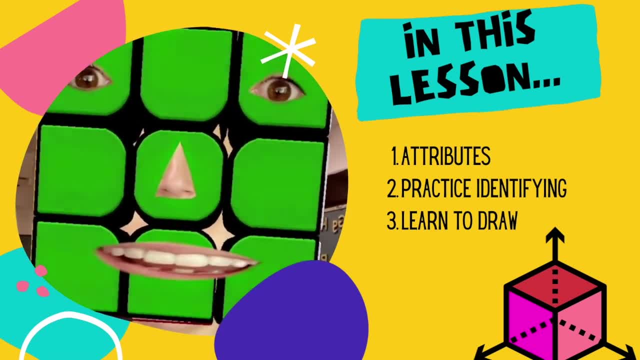 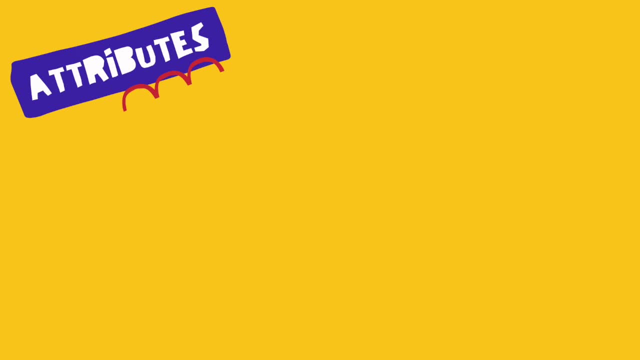 other 3D shapes. Finally, my favorite part, you'll learn to draw a cube. Make sure you stick around for that part. It's pretty cool. In order to identify or draw a cube, you must know the attributes that all cubes have. Let's start by talking about the faces of a cube, Remember. 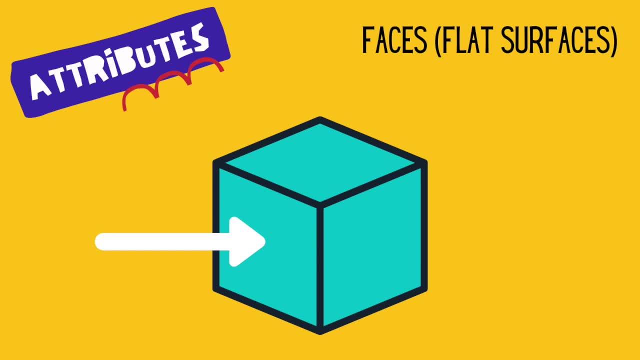 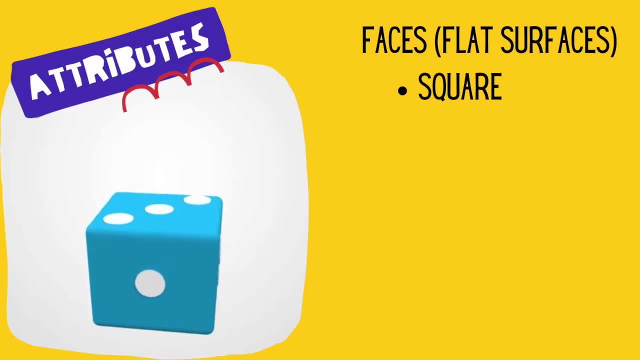 a face is the flat surface of a 3D shape. Each face on a cube is the shape of a square. Let's count the faces on this cube: One, two, three, four, five, six. There are six faces on every cube, and 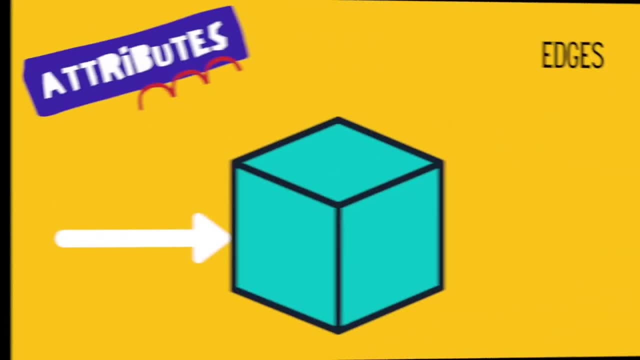 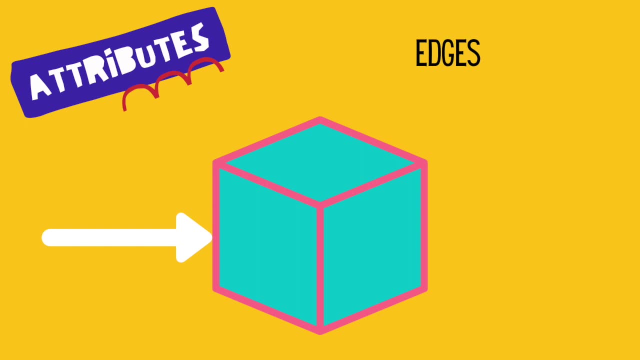 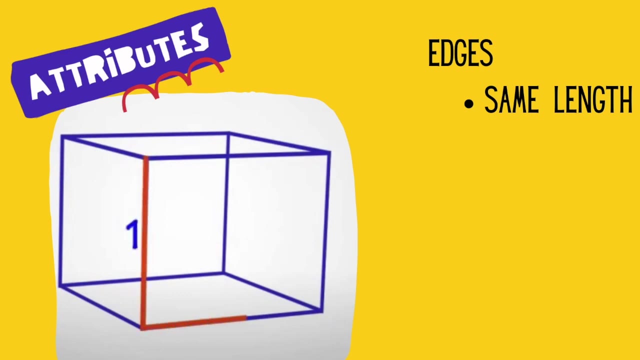 the faces must be the same size. Now let's talk about the edges on a cube. Remember, the edge is where the sides meet. All of the edges on a cube are the same length. Can you help me count them? One, two, three, four, five, six, seven, eight, nine, ten, eleven, twelve. 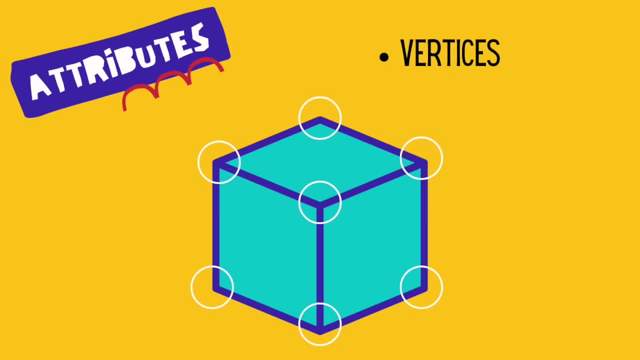 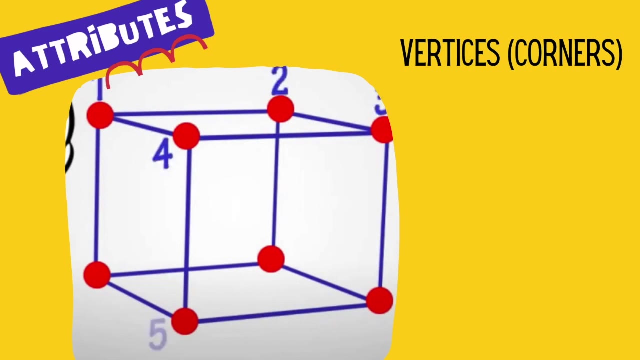 Cubes have twelve edges. Finally, let's talk about the vertices. Remember vertice is a fancy word for corner. Can you help me count the vertices One, two, three, four, five, six, seven, eight? A cube has eight vertices. 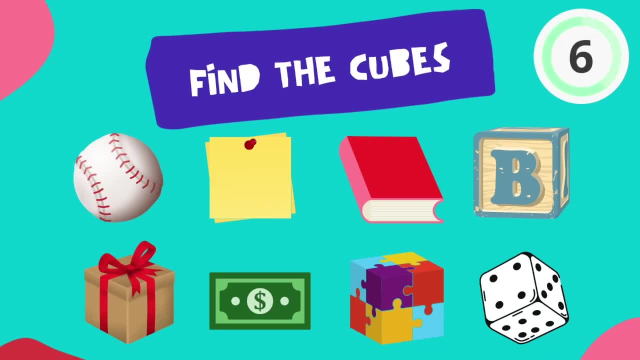 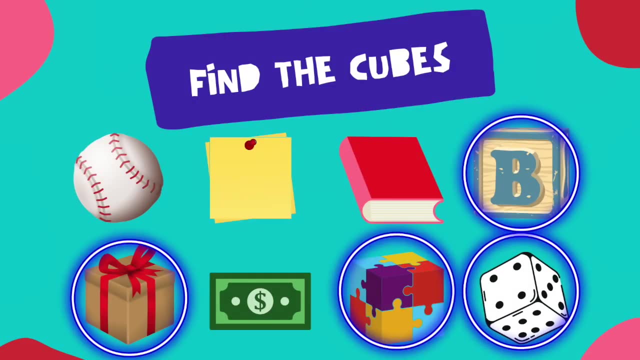 Now that you know what a cube looks like, can you help me find all of the cubes in this picture? Let me see one, One, two, three, four, five, six, seven, eight, 9,, 9,, 11,, 12,, 14,, 15,, 16,, 17,, 18,, 19, 20시�eptme quotations. 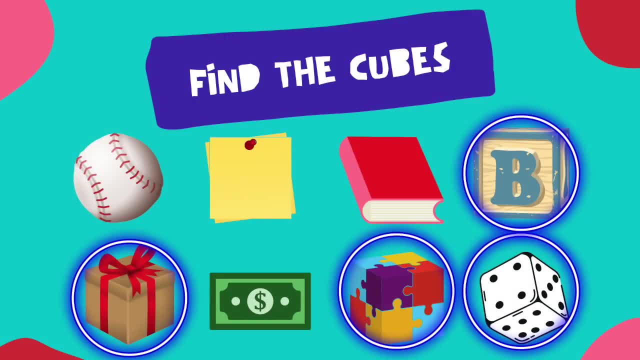 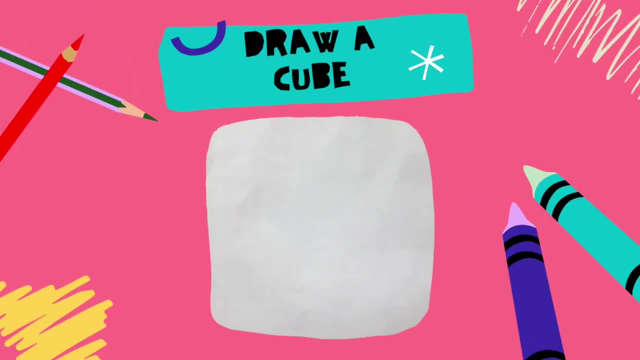 The block present puzzle piece and dice are all cubes. Het, probably you didn't get tricked by a piece of paper. A square is flat, A two-dimensional shape. Cubes are solid and have a three-dimensional shape. Now that you know what a cube looks like, it's time to learn how to draw them.